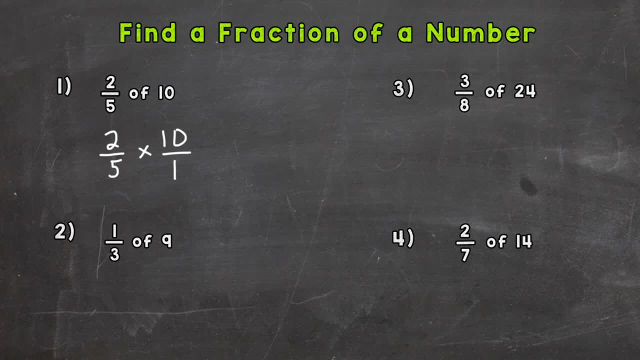 And it does not change the value of that problem or that number. So in order to multiply these fractions, I just go straight across: Two times ten is twenty. Five times one is five, So I get twenty-fifths. But I don't want to leave it as an improper fraction, So I need to do twenty. 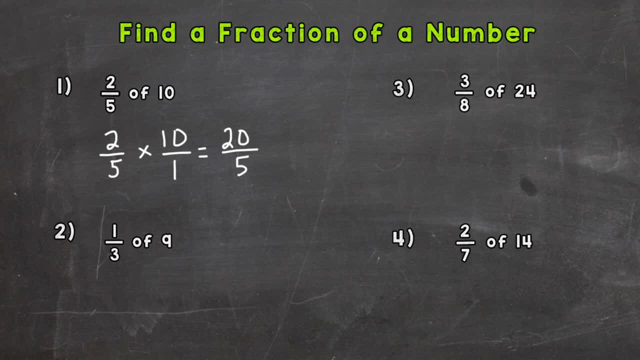 divided by five, and get this into a mixed number, or it might work out to be just a whole number. So twenty divided by five, how many whole groups of five can I pull out of twenty? Well, four, And that hits twenty exactly. so I don't have anything left over, And the answer to this problem is four, So two-fifths. 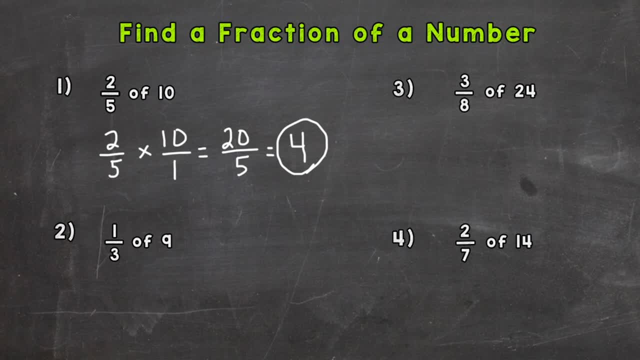 of ten is four. Let's go to number two, One-third, and then change the of. let's change it to a multiplication problem. Nine And remember, we can put our whole number over one. That way we have a numerator and a denominator. 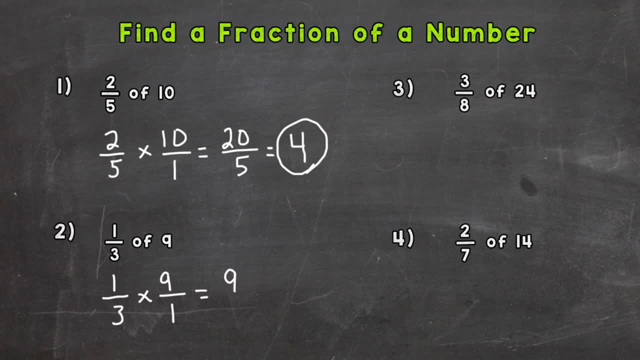 One times nine is nine. Three times one is three. So I get nine-thirds, And here I could do nine divided by three. How many whole groups of three can I pull out of nine? Well, three, And that hits nine exactly. so I don't have. 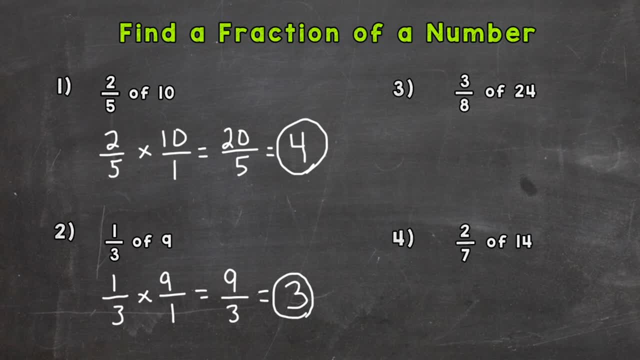 anything left over And my answer is just a whole number. So one-third of nine is three. So let's do number three here, where we have three-eighths of twenty-four, And I'm going to show you a different way to do number three now that we have the multiplication way down. 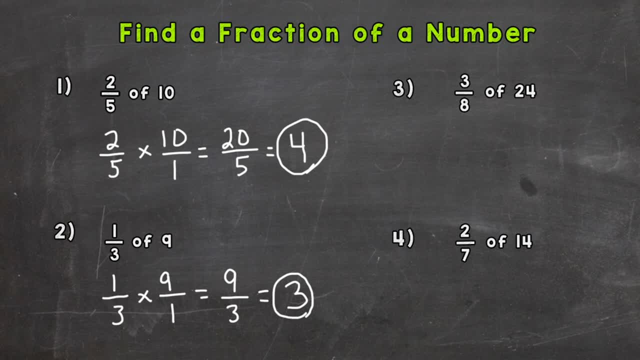 So I'm going to actually do the multiplication first and then the other way. So three-eighths times twenty-four over one. Well, three times twenty-four is seventy-two. Eight times one is eight. So now we get to this point where we have seventy-two over eight, and that's an improper fraction. 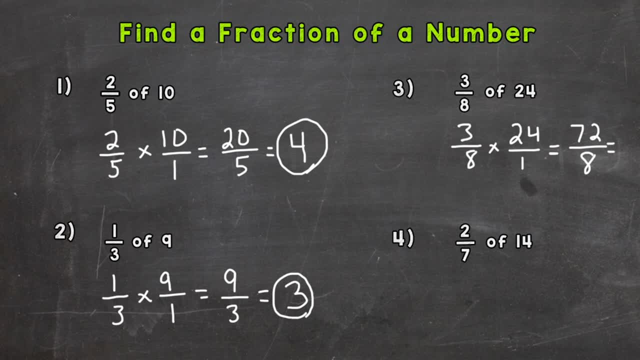 So we need to do seventy-two divided by eight and see how many whole-eighths we can pull out of seventy-two, And the answer to that is nine And there's nothing left over. So our answer for three-eighths of twenty-four: 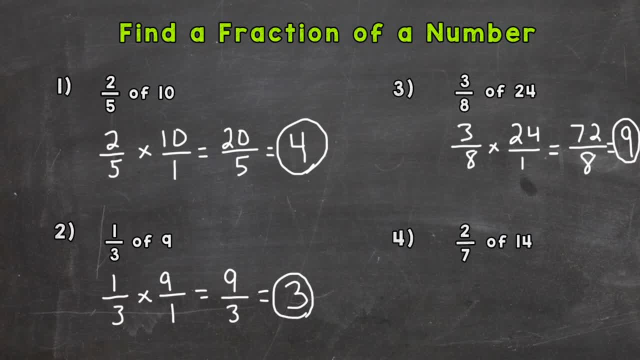 is eight. Now the other way we can do this is we can divide first. You can take twenty-four and divide by eight. So that would give us what one-eighth of twenty-four is. So we can divide first And then multiply it by that top number. 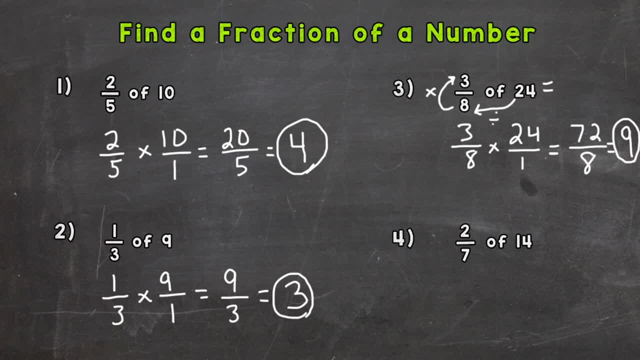 So again we can do twenty-four divided by eight. That would give us what one-eighth of twenty-four is, But we need three of those. So then you would multiply by three. So twenty-four divided by eight is three. Then multiply that by three to get three-eighths. 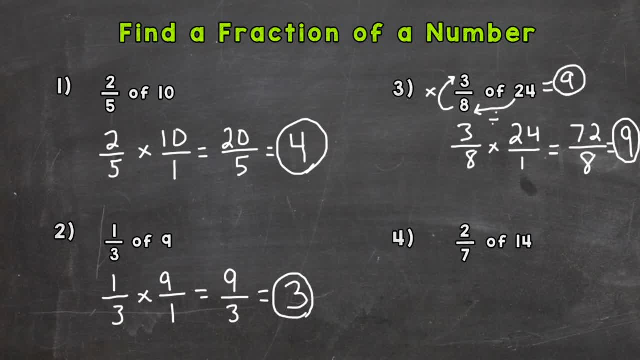 And three times three is nine, So we got the same thing. So you can divide first and then multiply by whatever the numerator is. So let's do number four, So we could do the multiplication way And we get two-sevenths times fourteen. 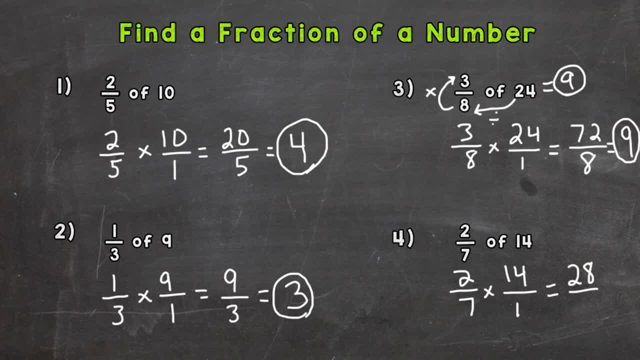 Two times fourteen is twenty-eight And seven times one is seven. We have an improper fraction. so we need to do twenty-eight divided by seven, which is four, And two-sevenths of fourteen is four, Or the division way. first we could do fourteen divided by seven. 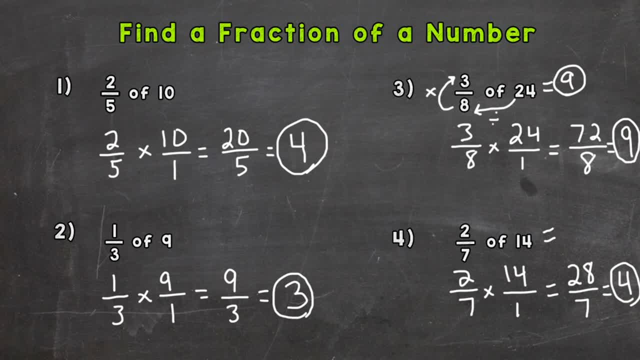 That would give us what one-seventh of fourteen is, And that actually equals two. Fourteen divided by seven is two, right? I take this fourteen, divide by that seven and then multiply by how many-sevenths I want, And I want two-sevenths, so I need to multiply two times two. 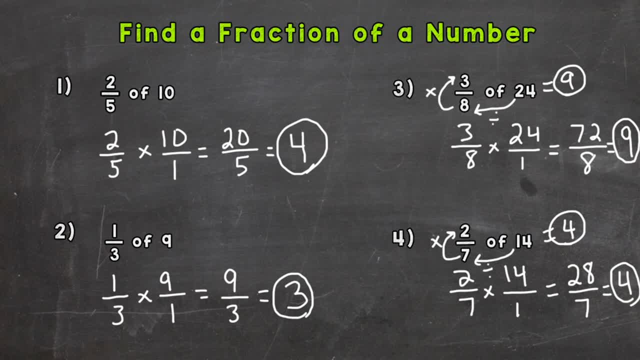 which is four. I get the same answer either way. So there you have it. There's how you find a fraction of a number. We can create a multiplication problem and multiply, Or we can divide first and find, for example, number four.